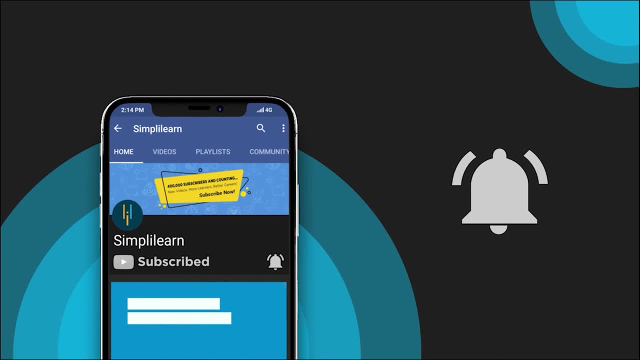 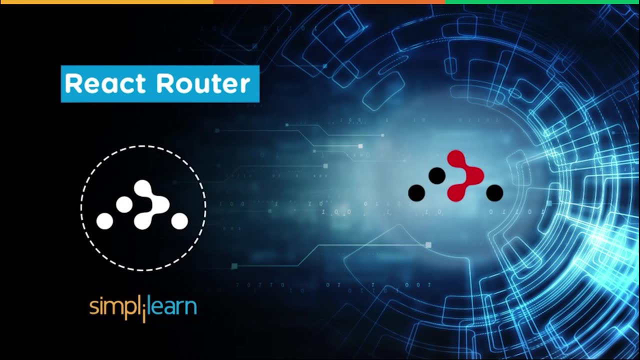 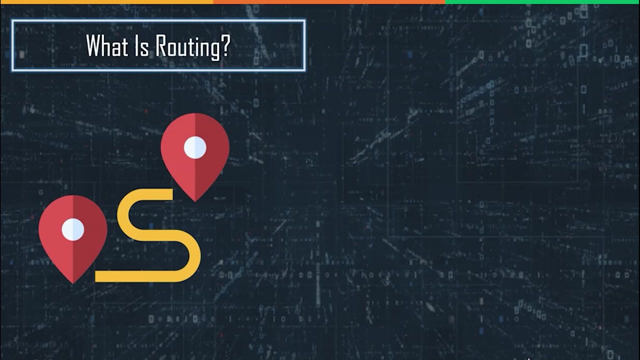 Hello everybody and welcome you all. So today we have a very interesting session coming up for this React, which is called React Router. So let's get started with React Router and see what it offers. So, friends, the first important thing about what is a routing, As we know, 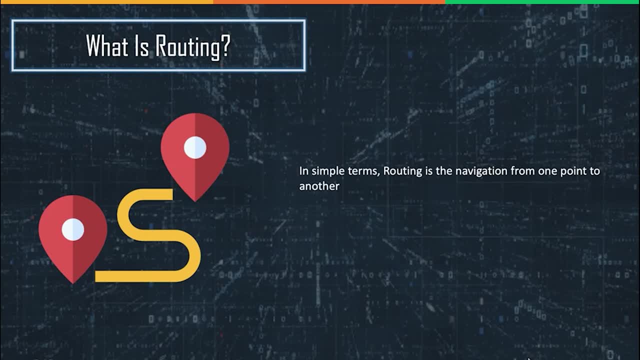 it very well. the routing is synonyms of navigation. Any application, whether you talk about multi-page application or single page application, it always requires a routing. Through this routing you will be making your applications, you know to be navigate from one part to the another part, like you have a call, login page, registration page and you have got a lot of links available. 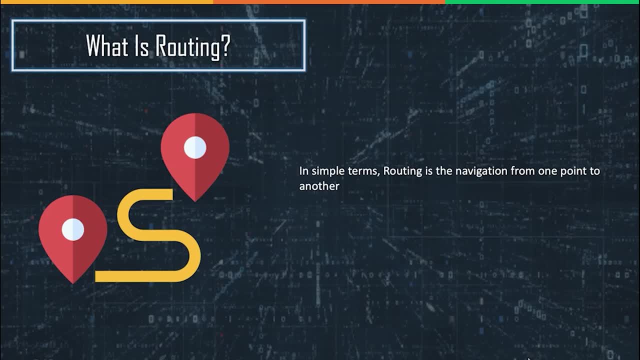 and when you click on those links, application will take you towards those necessary pages. but here in React Router you will get a lot of links available and when you click on those links in React these are component centric architecture. So here you will be having a components loaded. So, as we know, in a traditional web development, routing plays a very, very 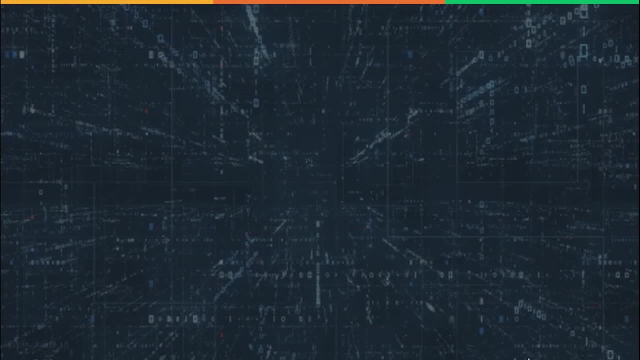 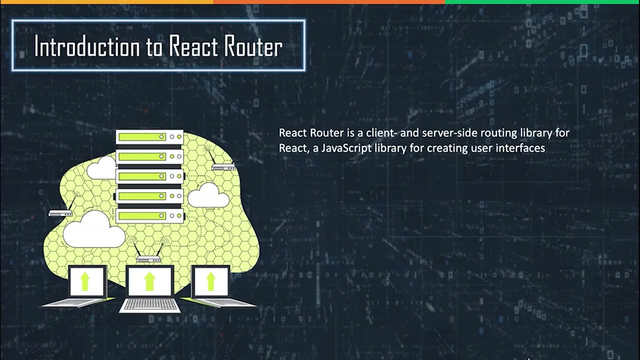 crucial role so that you can navigate through Now. React Router. So what is a React Router? So we know that React Router is a client and server side routing library provided by the React. It is a JavaScript libraries which is normally known for creating the JavaScript. 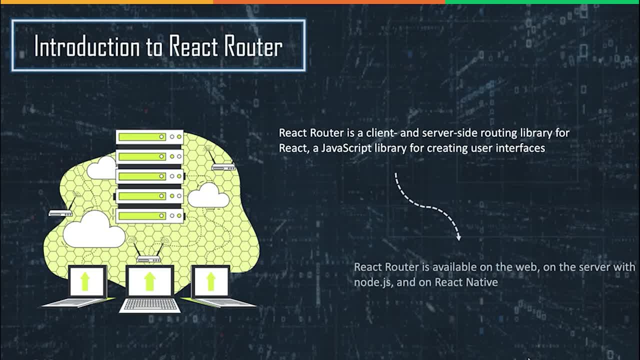 application. Now, React Router is not only a good application for creating the attractive user interfaces. Now here, the traditional React Router is available on the web and the server. so with using traditional Nodejs based application which is, you know, it is designed for developing a server side JavaScript based applications and all React native, which is 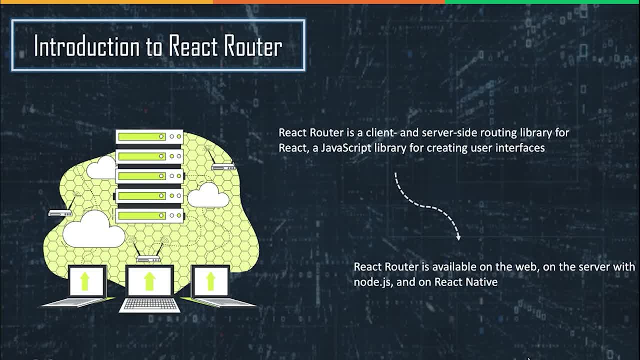 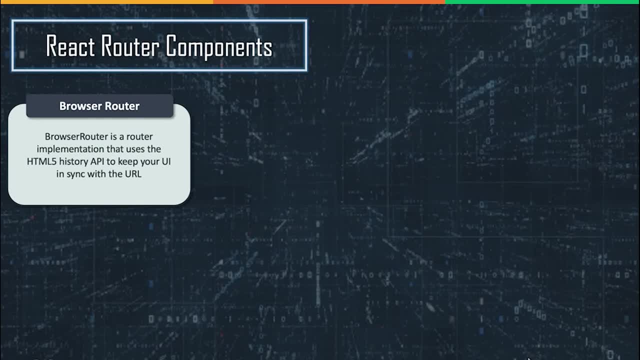 once again for mobile based environment, for React applications, router components, so browser router. so typically say the browser router is: this is one of the component, because react router comes with not many API. so here one of the API which is called browser router. so browser router is something. 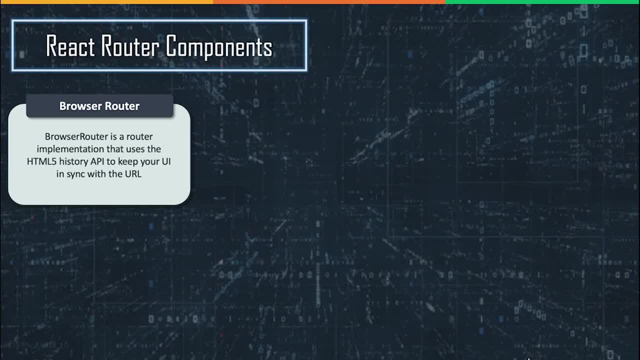 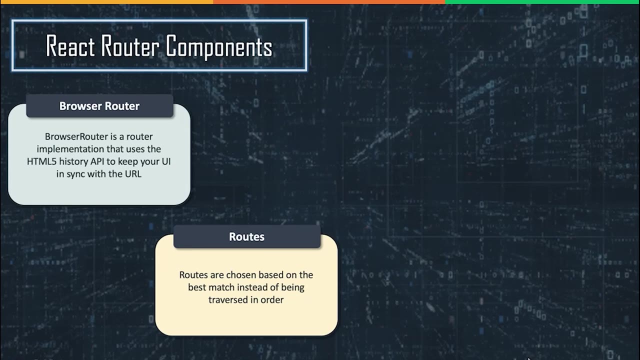 from where? okay, it uses the traditional HTML 5 history API, which is one of the main component, so it keeps your URL in sync with what you are navigating through. okay, so next we have a call: routes. so routes are basically chosen based on what best matches. you are providing it so that when you click on 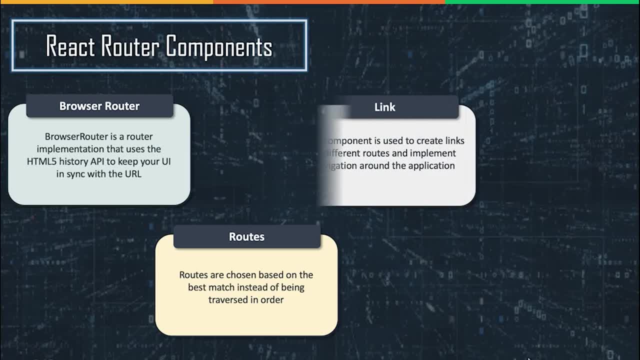 those links so appropriate route will get loaded for you- so called components. so now we have a call link, so the traditional link components are used to basically create a hyperlinks like a href, how we used in HTML pages. so two different from the traditional react app: the 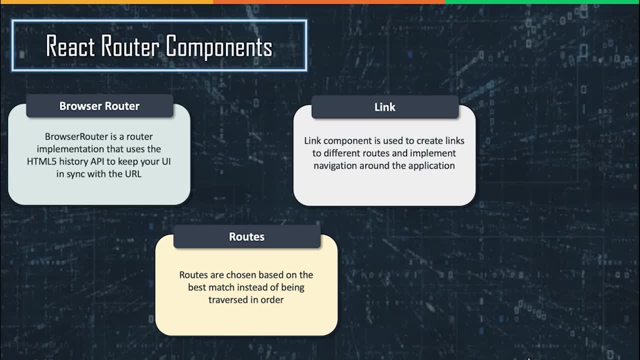 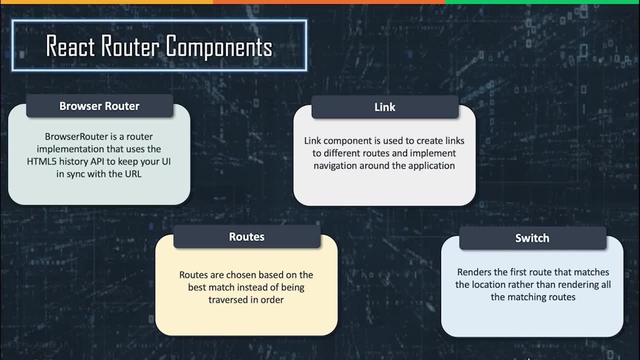 application, so it is mainly designed to focus on navigation throughout the applications. and now we have a call switch. so traditionally switch what it does? it renders the first routes and matches the location, rather than rendering all the matching out like whichever has come. it is like in typical switch case: whichever. 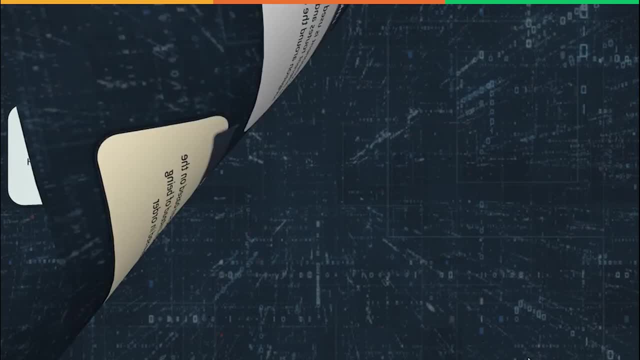 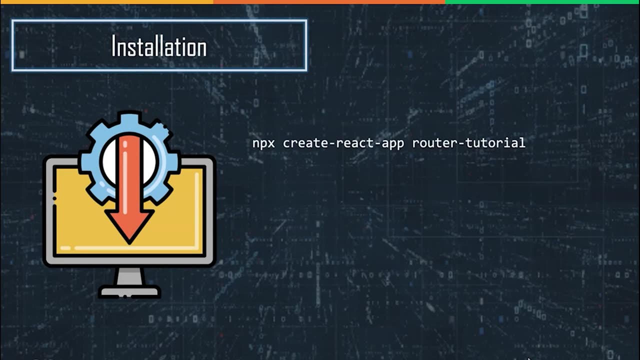 comes it, make it available and come out. that's how it provides okay. so, installation wise, you need to have first, you have to create the react based application. by using the application application, you can create react by using and px create react app. so create react app is a. 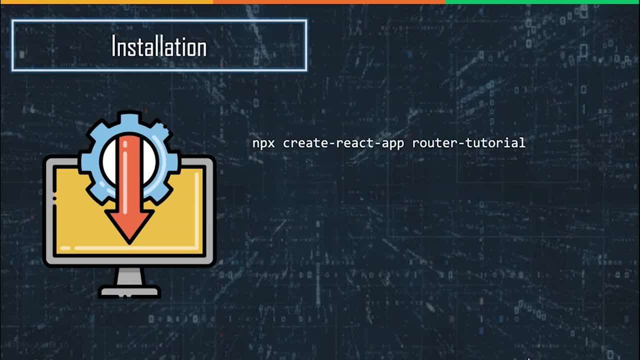 tool provided by the official Facebook and the router. hyphen tutorial is the name of the project. okay, so you will be using this command to create a new project for you and post that you have to install this particular dependency called react hyphen outer hyphen tom. so this dependency you need to install. post. 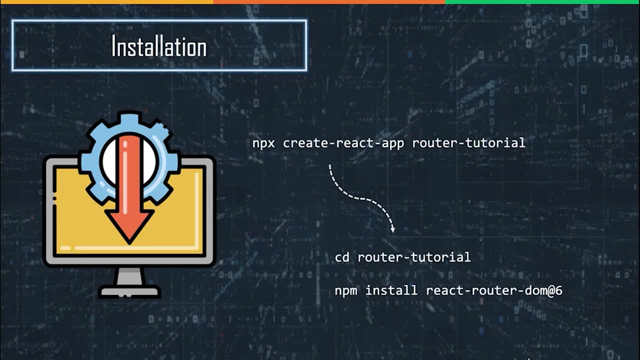 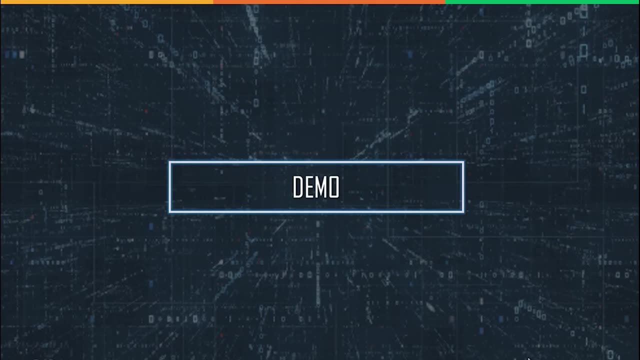 I would say the message is executed, so the ones. the first command is ready. then you'll be going inside this NPM install and then you say react router DOM. so this is how the steps are, and now we'll talk about demo. so let's get started. 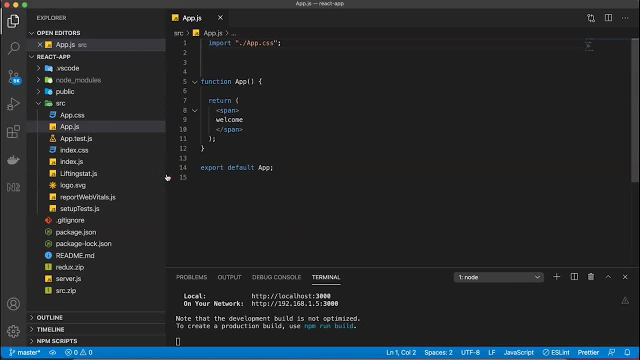 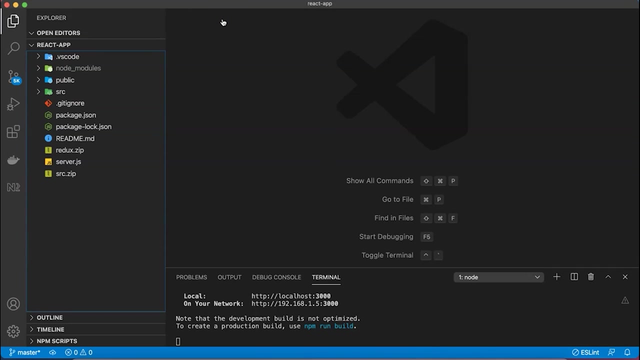 with the demo part. okay, everybody. so it's time to get into some hands-on. so I already have a project ready with me which we have created with using create react app. so my project name is react hyphen app and I would like to create a new router based example here. so the dependency regarding a react 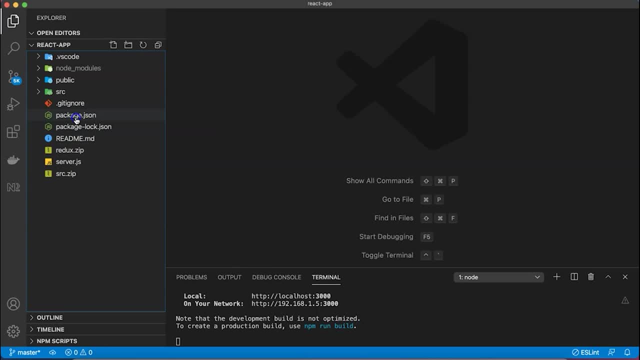 hyphen router, hyphen DOM is already installed. so if you see, this package, dot JSON react router DOM is already there in place. so we would like to start now developing those outer based example. so to make it happen, what we would like to start doing is we would like to create a new project that would 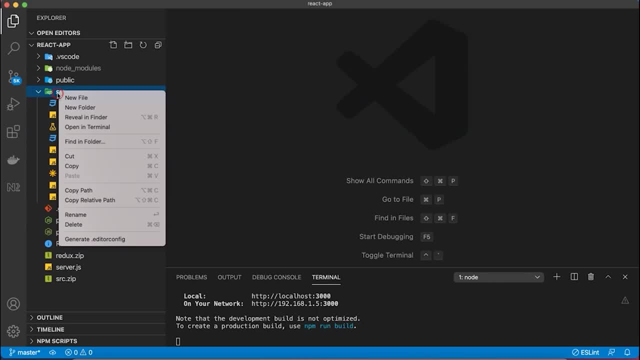 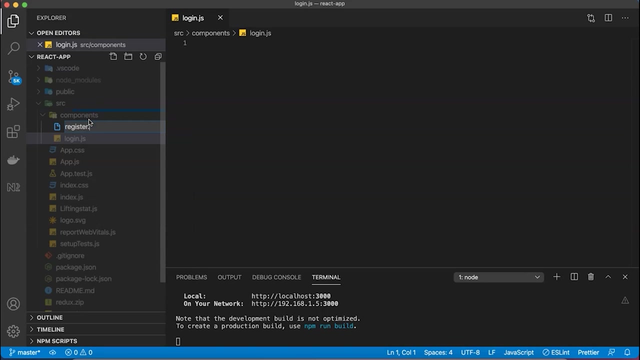 do is here in my src. we will create a new folder named components- okay, and inside this components we will create some file name called login dot js. likewise, we would like to create register user detailsjs. one more name call um yeah, portfolio. so we have got these pages already with me. 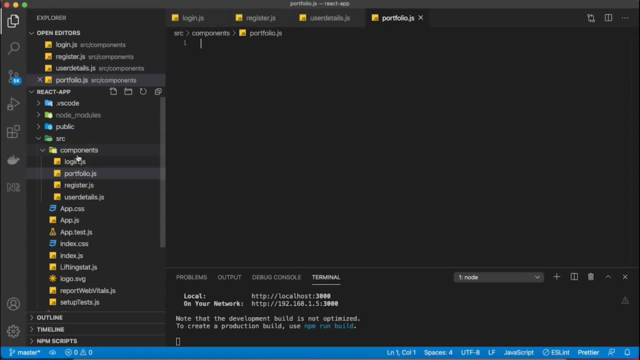 okay, out of which i want the first components to be get launched here. that is known as called a landing page. so here i will also create landing pagejs. so let's go back and create a new components here which will be helping us to move here and there. so first thing in my landing page, my component dot. 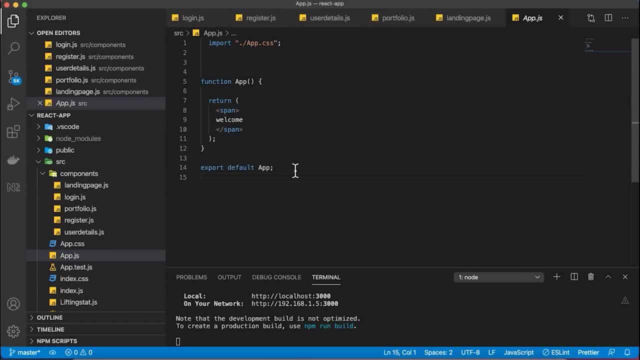 js. i have a call appjs, which is a base component for me. so, as i can see, this is how you go back and create a new functional component, so i just copy the same and here in loginjs we will paste it and give the name to login. 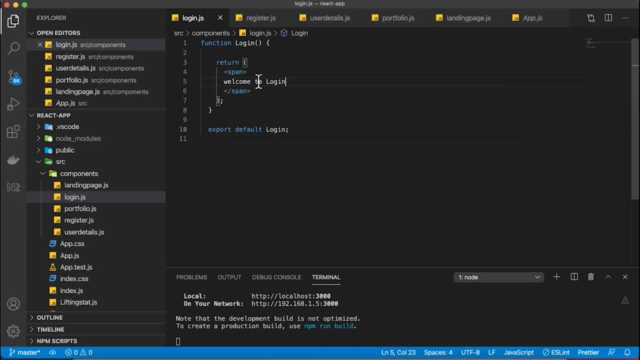 login and here we can say welcome to login. we just- this is my small component- i copied and i paste it in the portfolio and i paste it in the portfolio. so we will call portfolio: welcome to folio register. register login. we have got user details. looking for our user details. 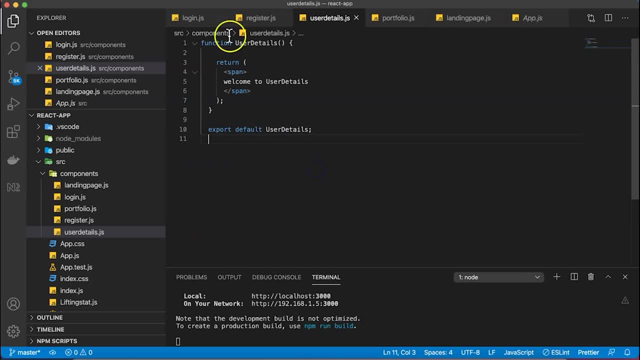 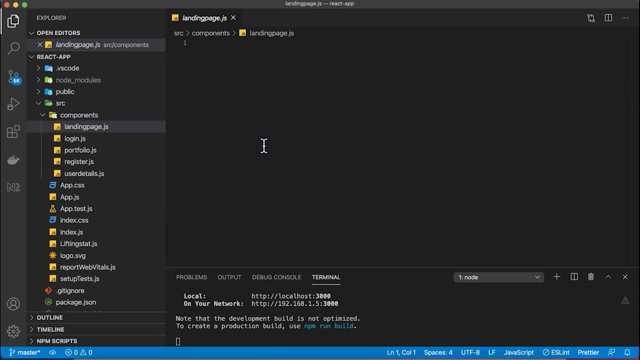 login, thenality default list. it algumas okay. so we have got these components with us. here are the some topics you can do to be a certificate. i will start with landing page first. so i would like to create a class-based component here. so import, oh, react from react now for default class. landing page extends component now render return. 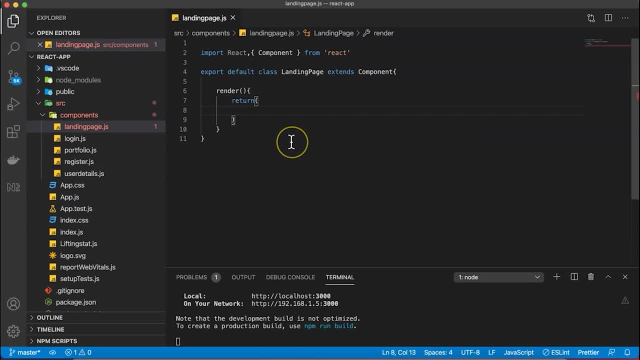 okay, so this is the one we're going to attack here. well, this is my component, which is available to me. so the landing page is a component which through which I will start working on. so I can say so here: I want this components to be available outside, so what I will do is this landing page in my 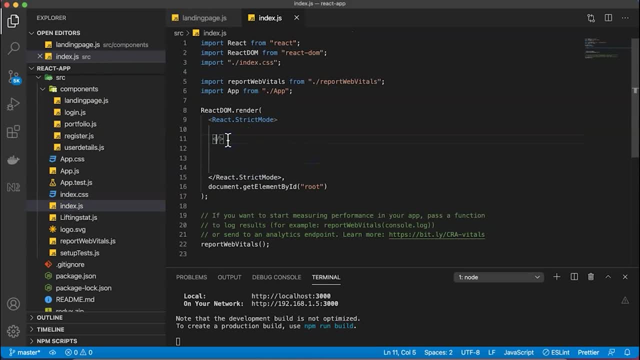 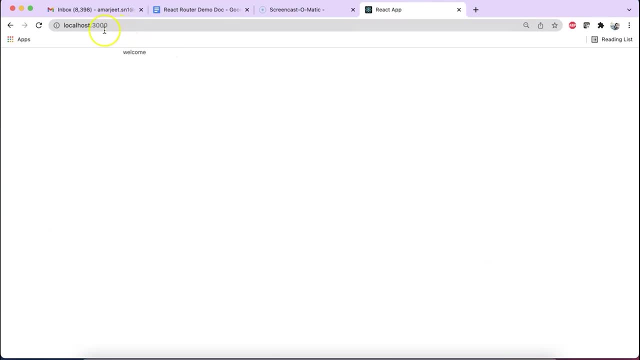 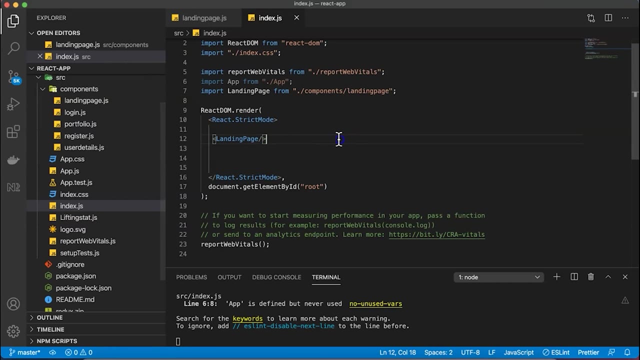 indexjs. I will make it as the first component to be launched landing page. so when I start my application, I should see here: okay, welcome to learning is coming up, perfect. so this has become my first component which I want to launch and furthermore, we would like to add few more. 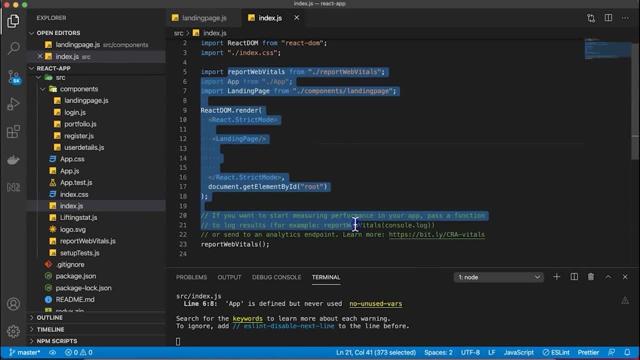 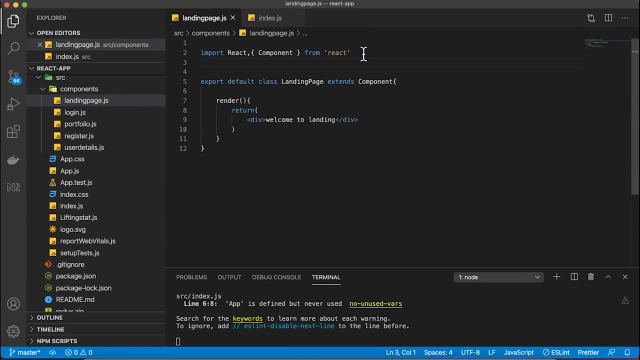 components here. okay, so in a previous program we have seen how to create a multiple components and how we can make one of the component design learning component. now it's our next program where we will be enabling the routing into our code. so in our learning page we would like to create some more dependency while saying import. 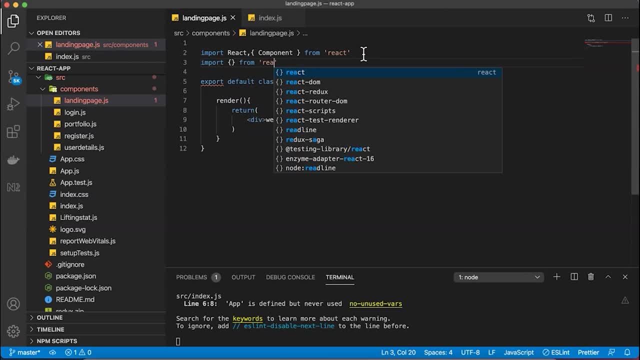 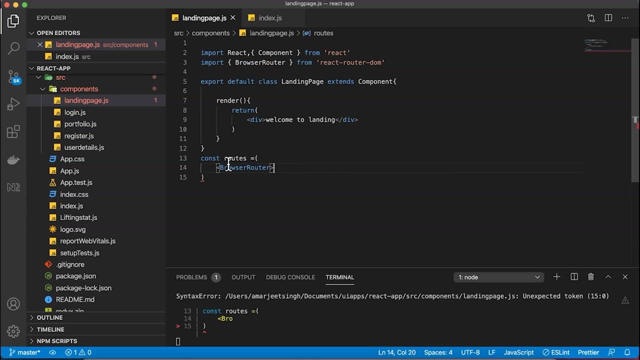 from react-router-dom. so we will be choosing those dependencies one by one, but from there we want to start working with cons routes equal to first thing, as I discussed with you, that is, we would like to start with the browser router. okay, so from this point onwards we would like to start with switch. as you can see, they are taking. 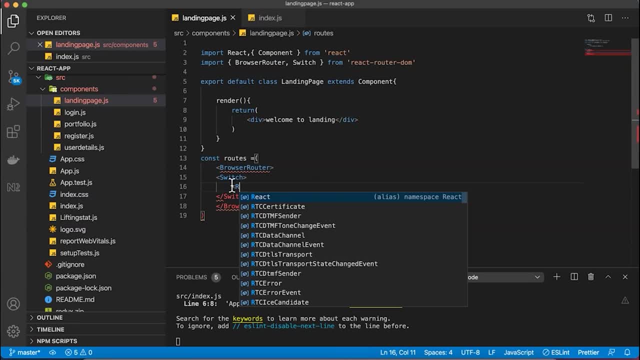 from the react router down after the switch. we will say route. okay. so here with this we will like to say the navigation path. we say path equal to. if it is login, then which component I want to launch? so we can say component here and say c, small component equal to. 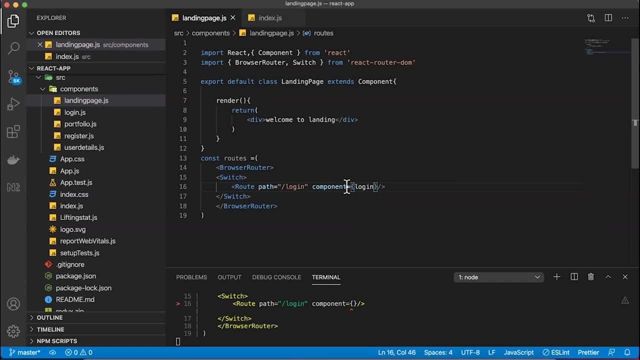 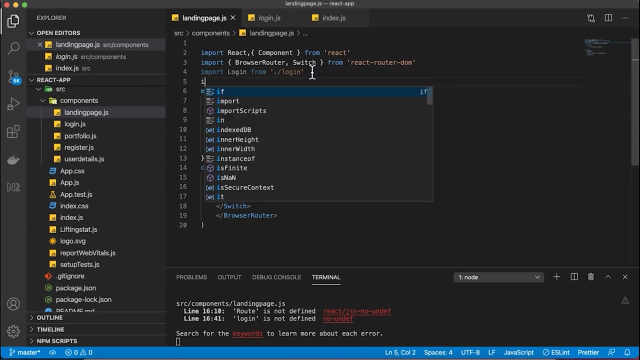 okay, it's not loading, so we can say import. and since I want to launch the component which is at type of login, so we can say import from login, so if you see here they were called login, so we will be using this login only. okay, so this is my login component. likewise, I will say: 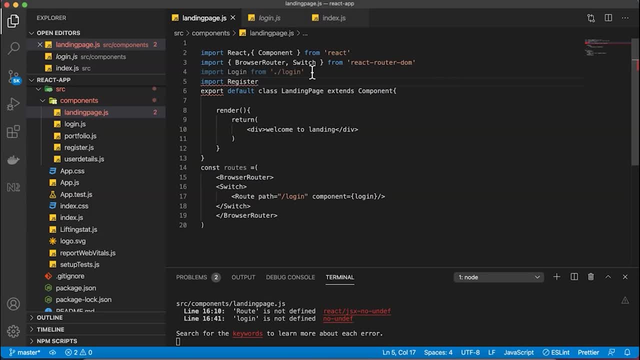 register. so here we would like to say login, and in a similar way we also want to have the other registration. I copy the same use: this register, register. so this is how the components are used here. okay, well, these are the quick to components we have created. one is called login and second for register, after that what you will. 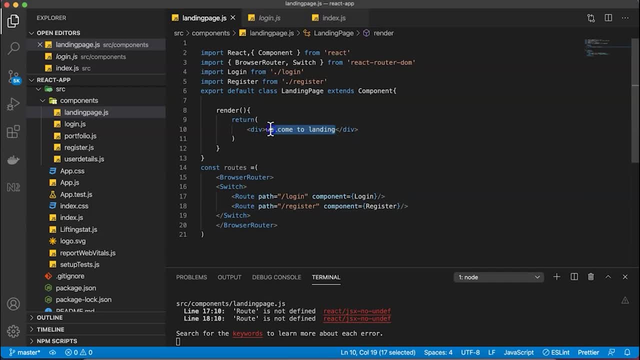 be doing this: routes, you will be adding it and assist div tag from removing this landing page and here we will give the name: call routes. that's it. so once this route has been given, now it's time for us to see what it differs. so, landing page or sorry? we have a register. we have a. 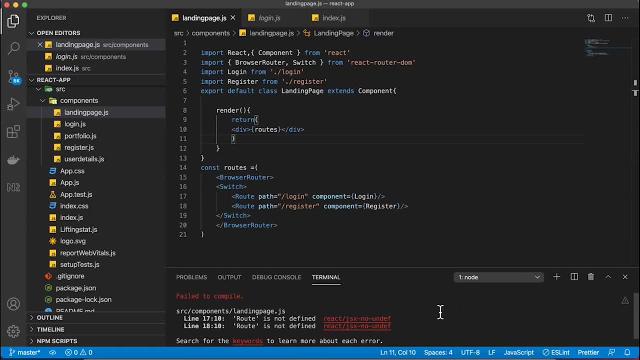 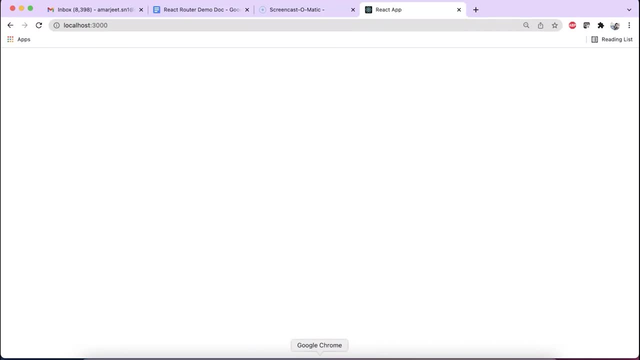 register also. so say: route is not defined. so what we can do? we can also import the route from this page. now let's go back. okay, nothing is shown. so now we have to manually type by saying login. you can see I've got this message called welcome to login. now let's see register and there 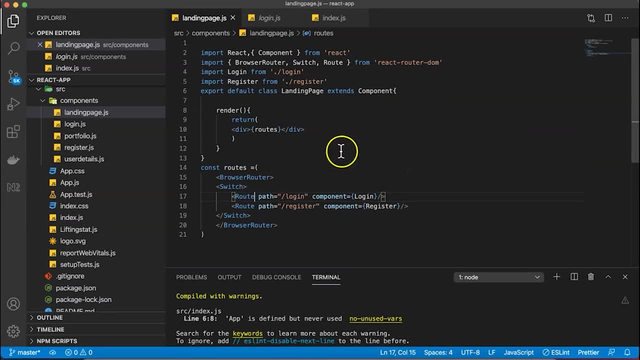 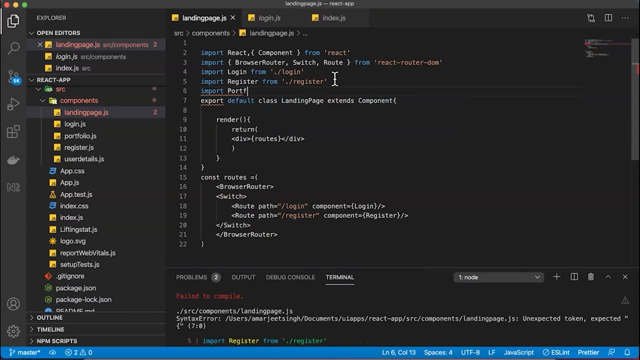 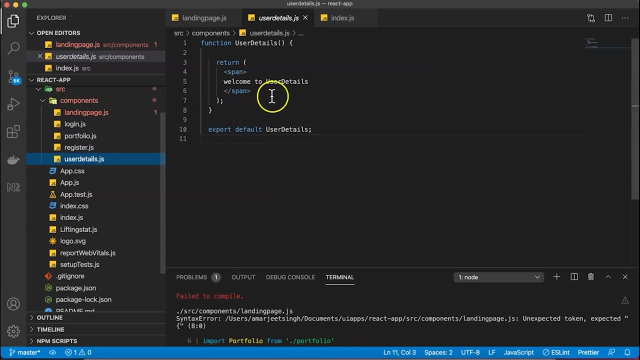 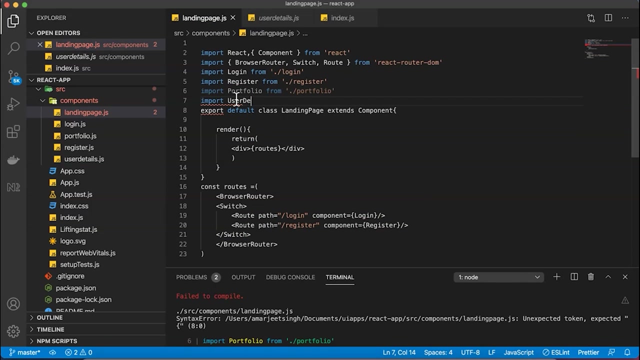 we go register. so two components are loaded correctly. now we would like to import two more: import portfolio portfolio, okay. and last we have a call, a user details, import name, call, user details. so we got user details. let me copy these two. so register portfolio. so this is how our 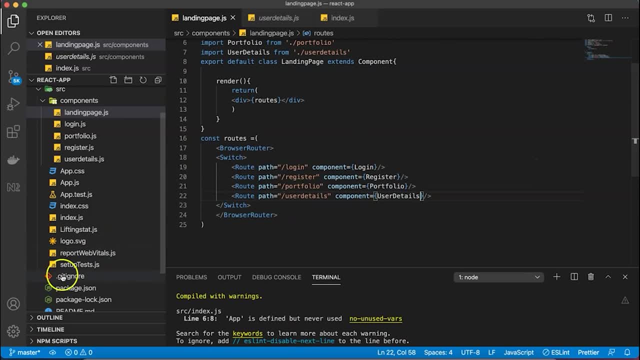 components will come to work are. so now we can see all the registered successfully. well, in our previous program we have seen we were typing those words manually into our browser, but in real time this won't be a solution in a real time. you would like to make this example by clicking on a hyperlink. you would like to make it. 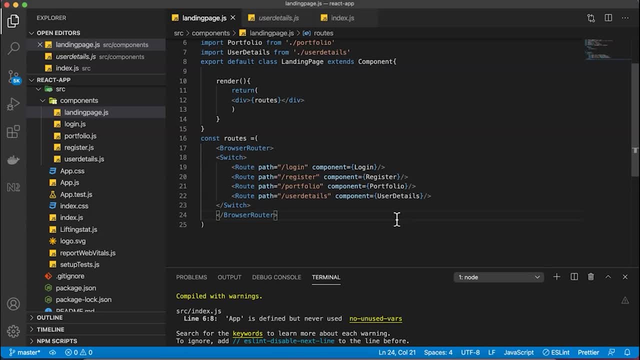 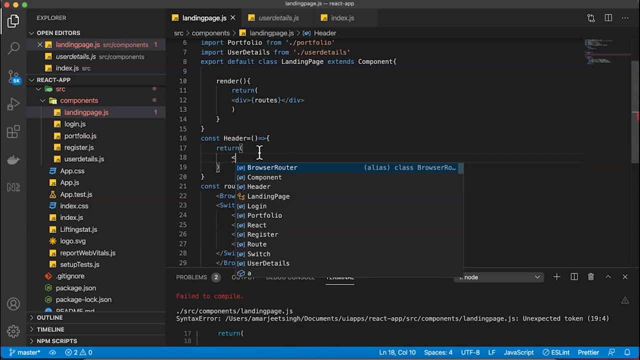 possible. so how you'll be doing this. so to make it possible, what you will be doing is like here itself, you create a new component called header. okay, so this is how you're going to create the new component called header. okay, so within this, you're going to add the new. 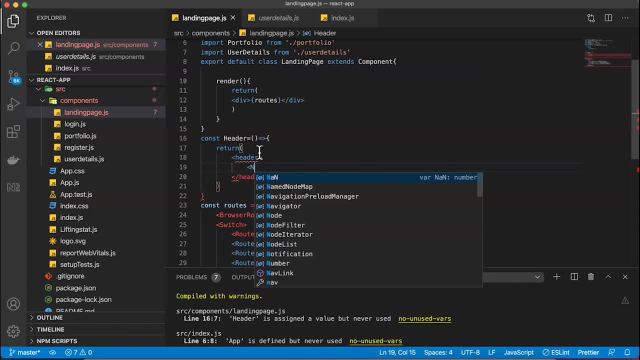 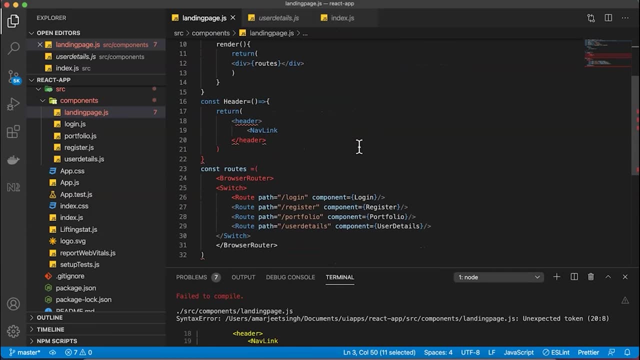 component called header. within this you will be using navlink, which is once again the tool provided by react, to which you can create a hyperlinks. so this is the navlink for you. so, within this navlink, you will provide the option, like in, to equal to login and along with this, you will also provide the 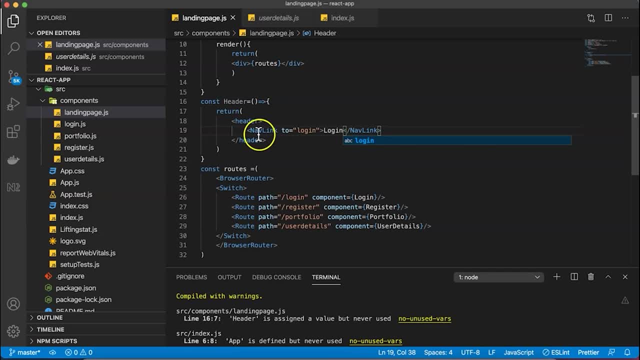 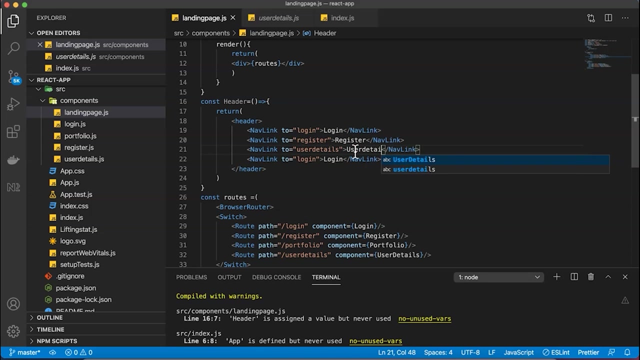 option like in to equal to login, and along with this you will also provide the option like in to equal to login, and along with this you will also provide the name. so here I say log. let me copy the same login register register. we also have called last. we have called: 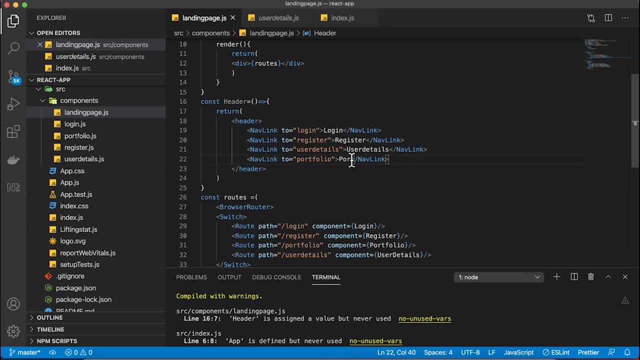 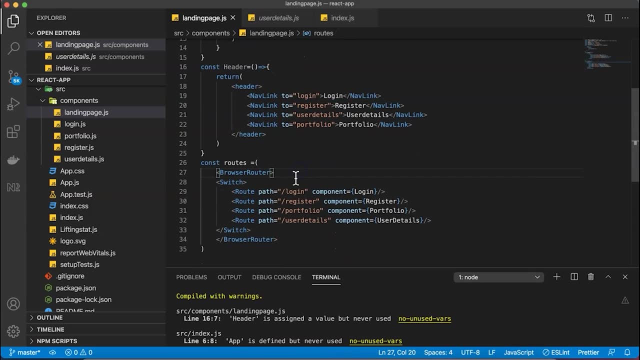 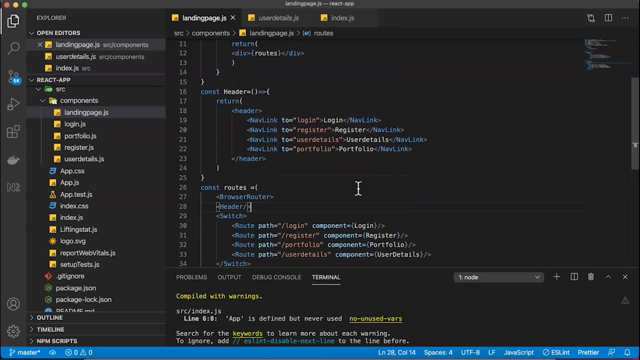 So this is my component, which is available to me, and this I would like to use within my application. So here, after this browser router, we would like to add the component called header. here, That's it. That's the only thing we need to do now. 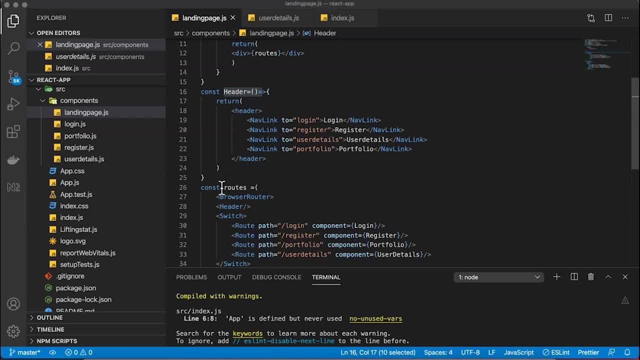 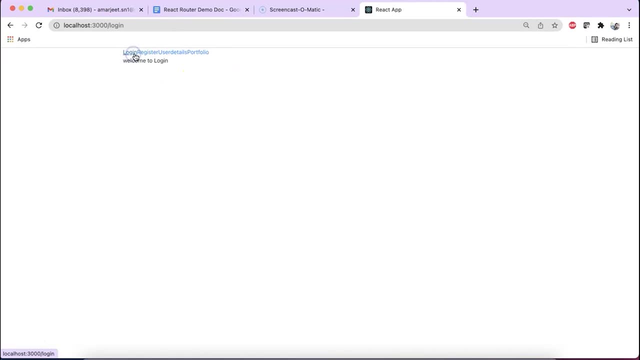 So this header component is now the part of routes, and let's see how it makes a difference. Now you can see very clearly it is having those links with me, and now, when I click on those links, you can see how these are easily accessible to all of us. 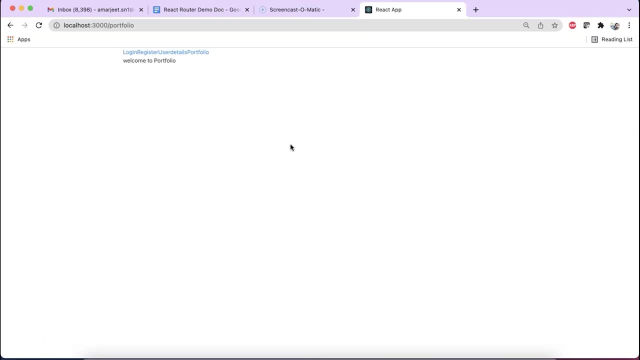 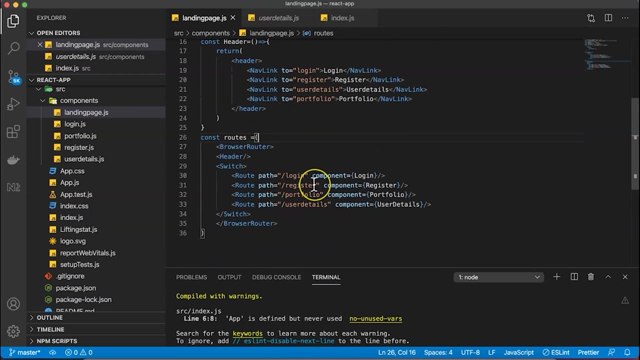 Okay, so these are the links which are available to us, through which we can make our components simple and easy to access. Okay, One more thing, we can do it here, and what's that? This component, whichever we are talking about. okay, This component we can attach to one of my base component when my component start it. 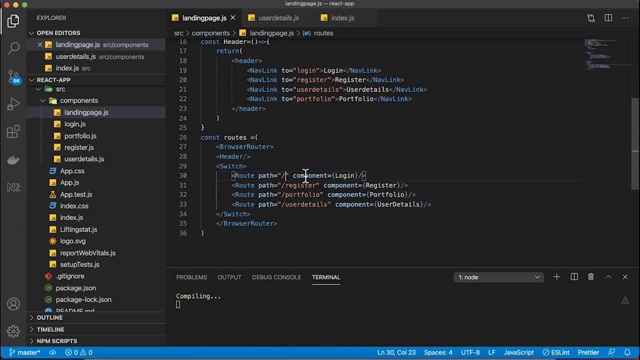 should work automatically. So I can do one thing: let my login component to be the base component for me. So in order to make this possible, I need to write one more tool here called exact equal to. Okay, That's it. 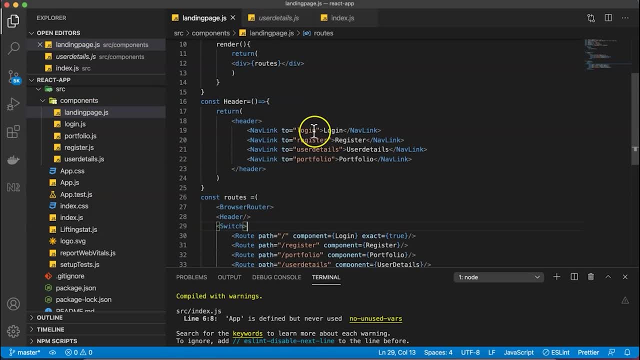 So here I will use the exact equal to true, And here also we have to use the same. So here we would like to add one more property here, Okay, And it will say exact equal to true. Okay, What I would like to use? exact equal to true. 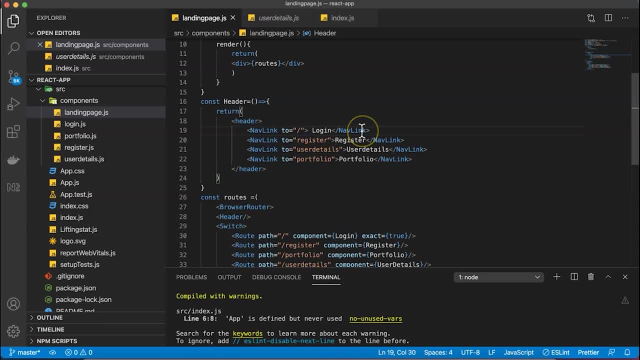 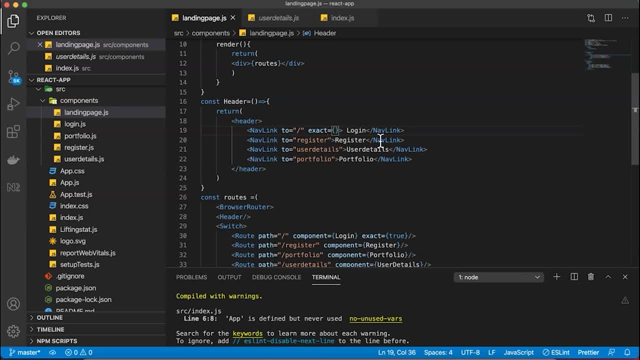 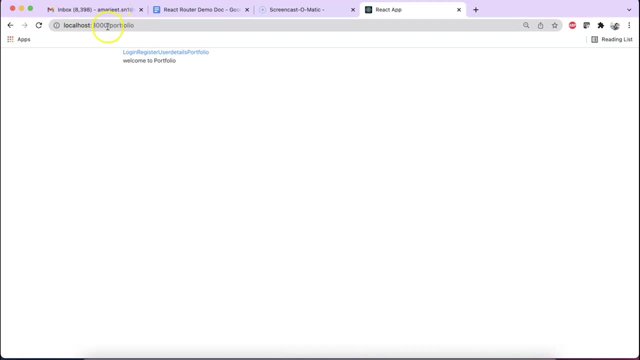 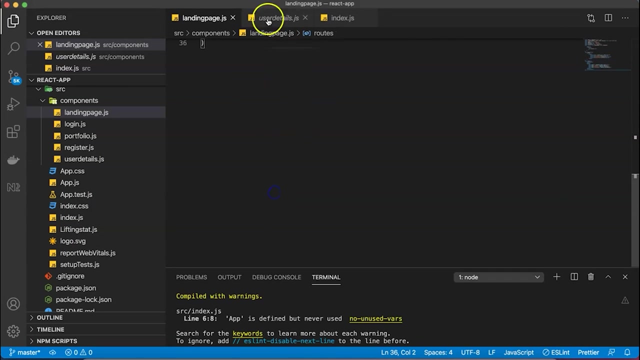 Bye, Bye, Bye, Bye, Bye, Bye, Bye. your job is done. now let's check. and now you can see the by default login page appear, because the login is in root location and that's how your URL works. okay, everybody. so in the previous examples we have seen how the links are. 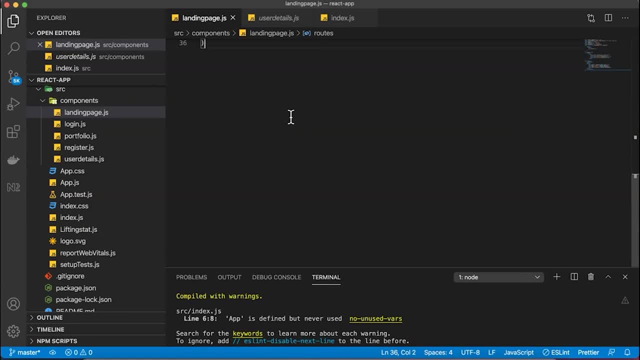 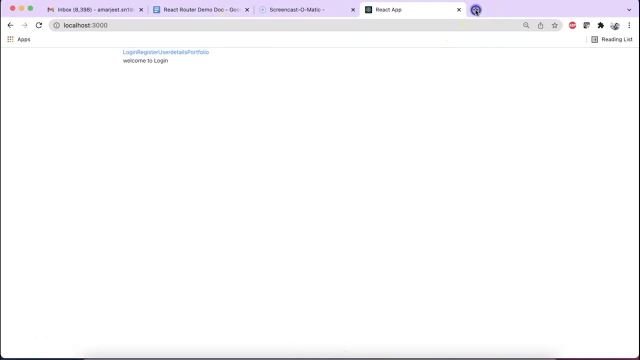 working. but these links are all internal links. but what in case if I want to go to the external link? so let's try to understand that point. so here let me try to open up. I'm opening up, simply learn link and clicking on this, the URL is: 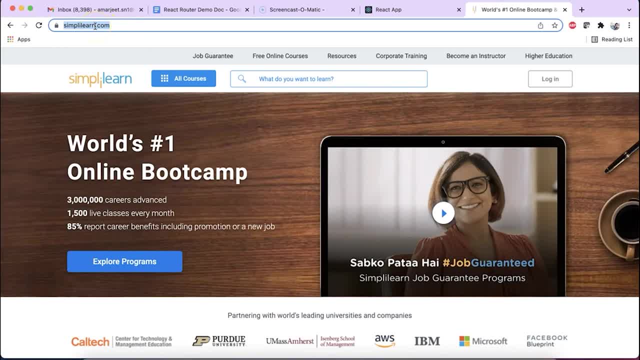 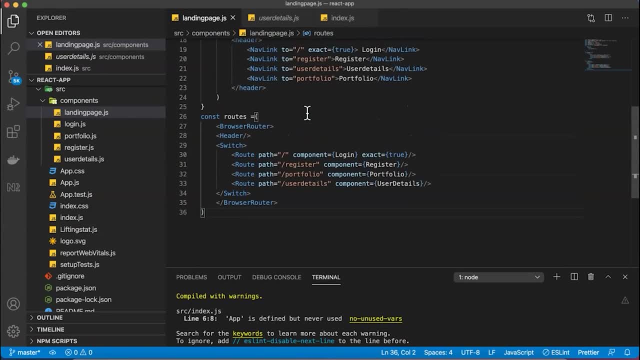 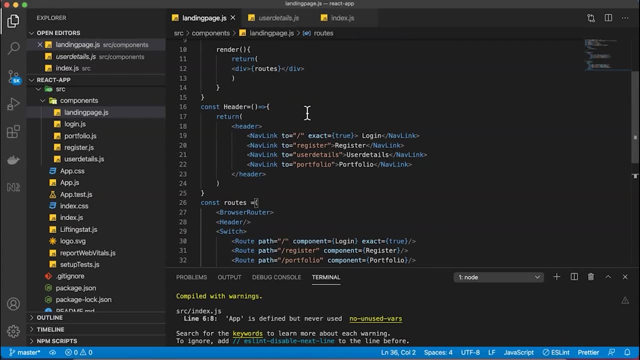 right now, HTTP simply done. calm, that's a link which is available, so let me try to copy this link and here, if you want to go to that location, so what do you need to do now so to make it possible? here I can just make this another nav link. copy the same. 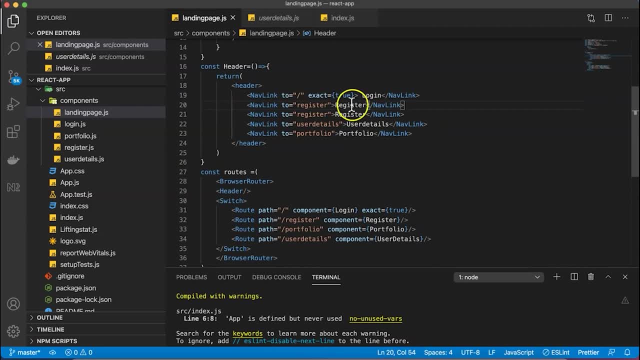 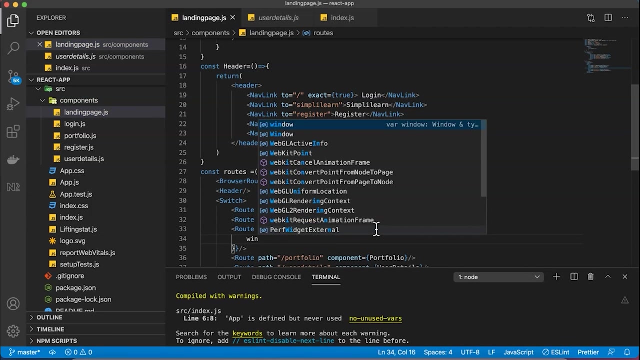 and I give the name called simpler, and, and here I'll just copy the same name. okay, so now it is asking me for it because I do not have any component here right now. so here what I will be doing. instead, I'm making it as a blank, ok, and here I want to give window dot location. 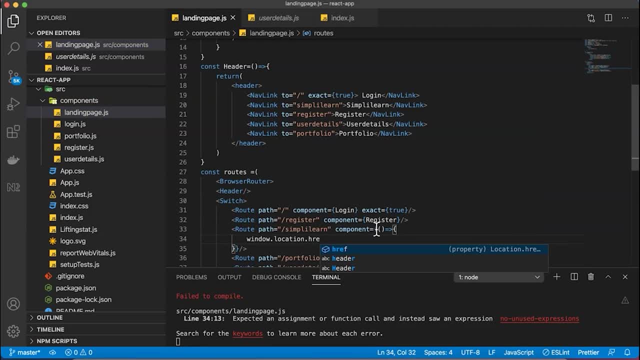 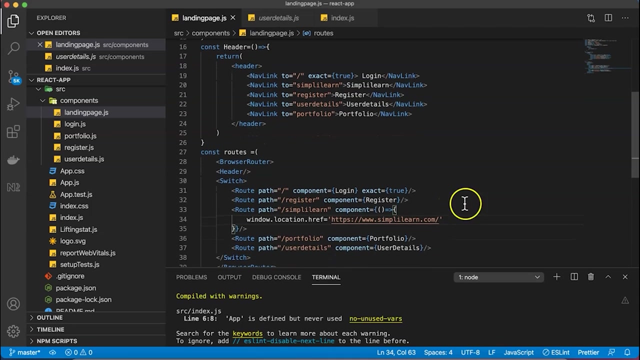 talk about to give window dot location. okay, I just handful of names here, okay, and here I want to give window dot location href equal to the website which is available. okay, so that will be the link which I am providing it now, and after this link, what has been provided? I'm saying return, that's it. okay, so that will be. 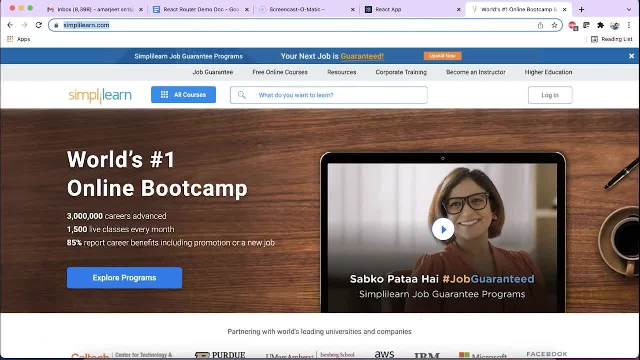 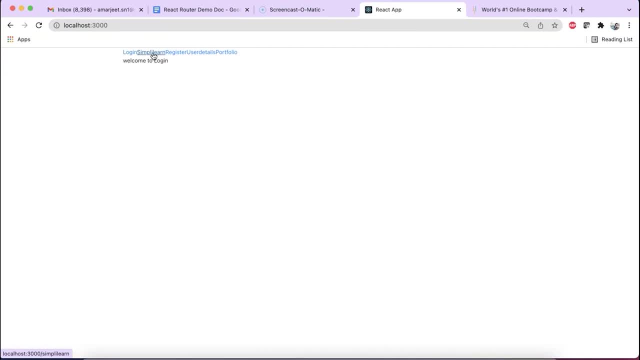 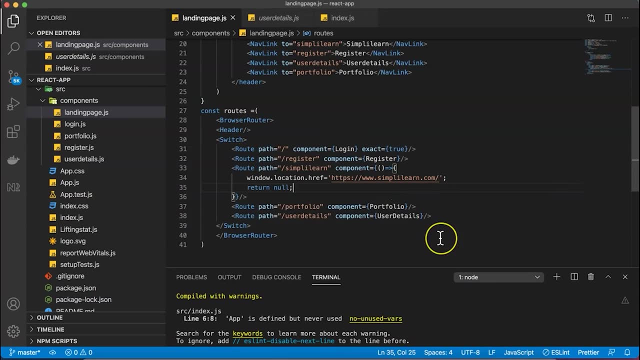 the link. so I'm saving this and going back to this location now so you can see we have a call simply done the moment I click it here, so it will somehow try to take me towards where this external website, the one which we are actually looking for. so I'm going to click on that and I'm going to 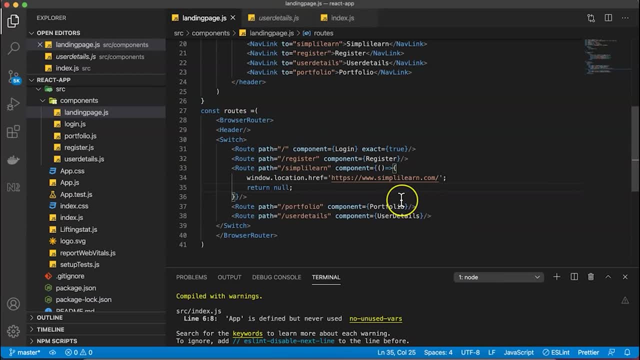 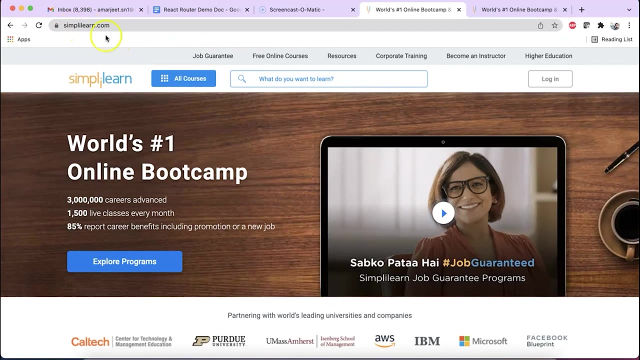 forward for okay, so this is the way through which you can basically make the application accessible outside. so if I just go back to my browser and refresh this, I click on simply learn and you can see now it took me to an external location called simply learn dot-com. likewise, 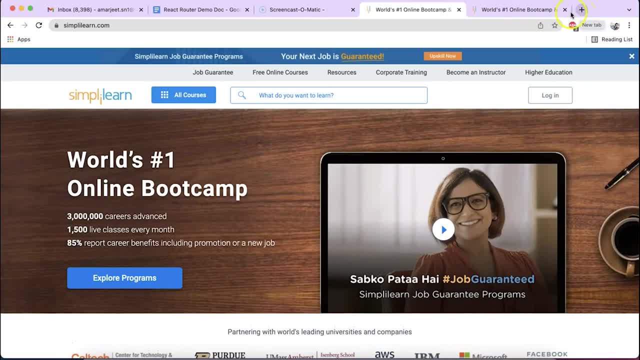 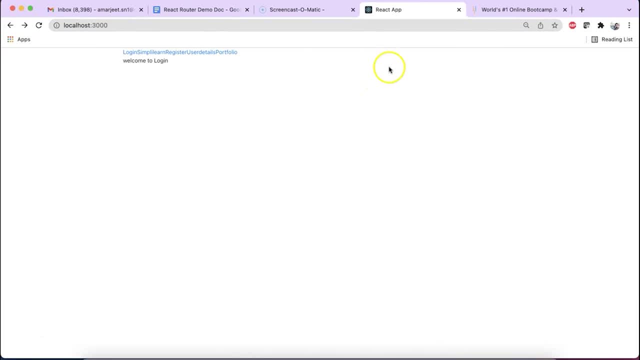 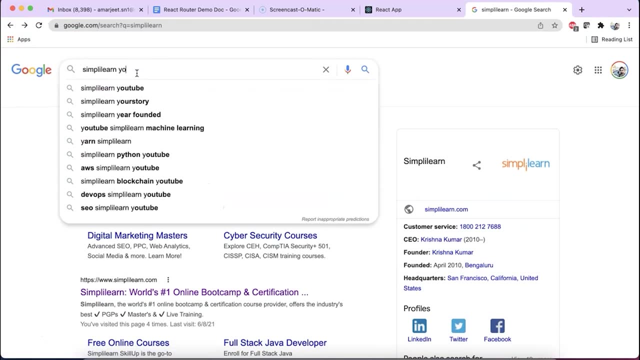 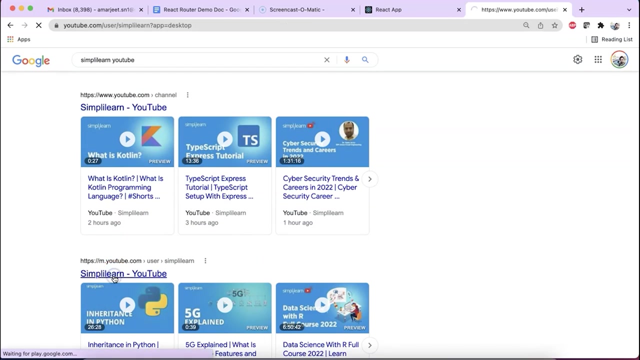 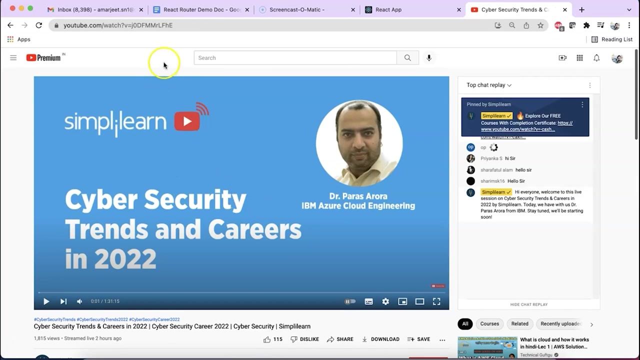 if I just go back and open the simply learn as a YouTube channel, also just say, okay, simply learn YouTube. so if any of the, I would say the link which is available. like you can see, right now we have multiple websites, so if I just click on anything, suppose,